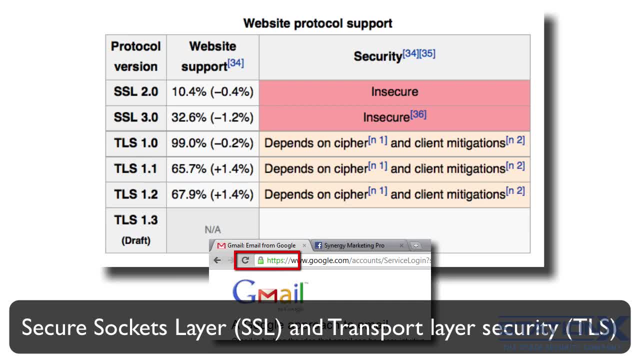 in the URL of a website, such as here. But TLS can be used with any other protocol that you want to use, like FTP or virtual private networks. It isn't just used with HTTP and for web browsing. TLS is very important for internet security and privacy because it is: 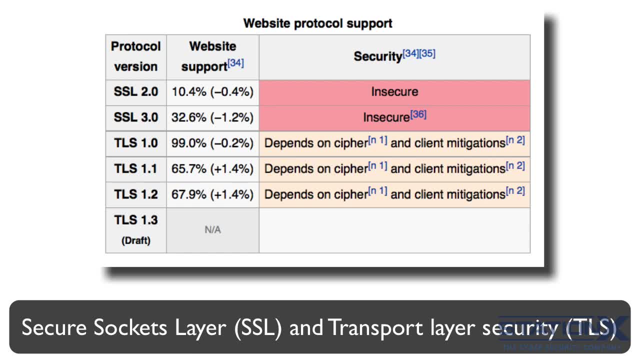 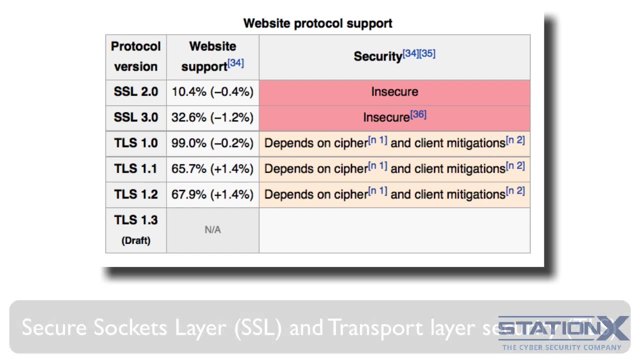 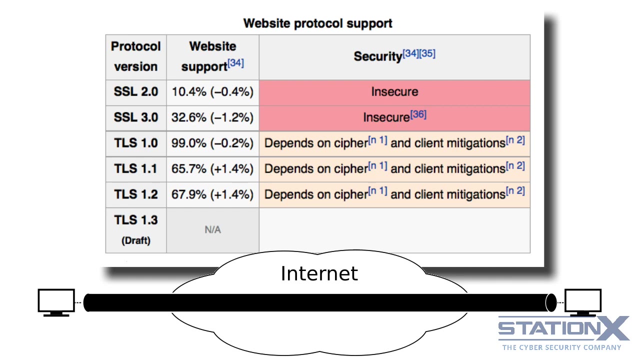 the most used method of encrypting data on the internet. TLS provides privacy because it encrypts the data, and data integrity because it uses message authentication codes or MACs, when communicating between two applications. So, for example, when you're working with a web browser, the application communicates with your online bank. their application, the communication. 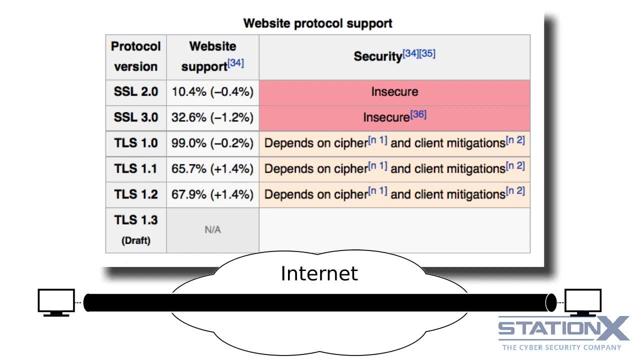 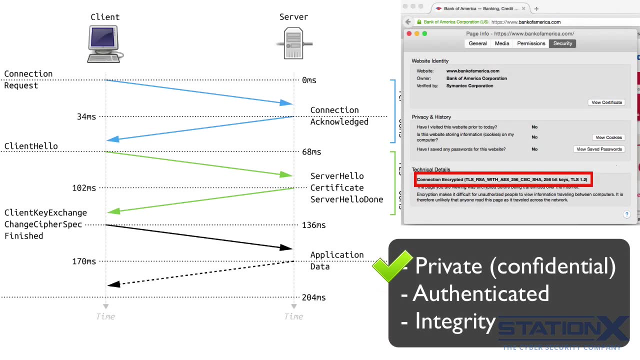 is encrypted from end to end, from your application to their application, using TLS. TLS supports the security services of confidentiality or privacy, authentication and integrity. The connection is private because a symmetric algorithm such as AES, which we've discussed, is used to encrypt the data transmitted. 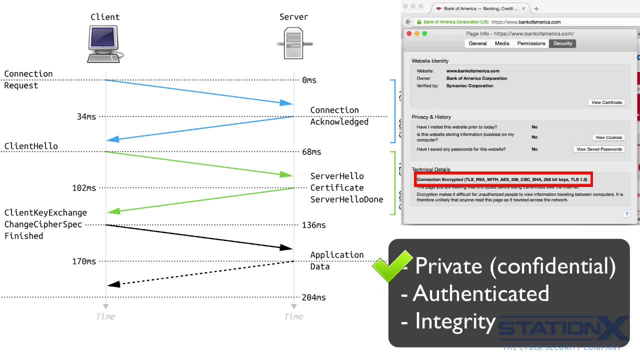 The keys for this symmetric encryption are generated uniquely for each connection and are based on a secret negotiated at the start of the session. The server and client negotiate the details of which encryption algorithm and cryptographic keys to use before the first byte of data is transmitted. The negotiation of a shared secret cannot be read by eavesdroppers. 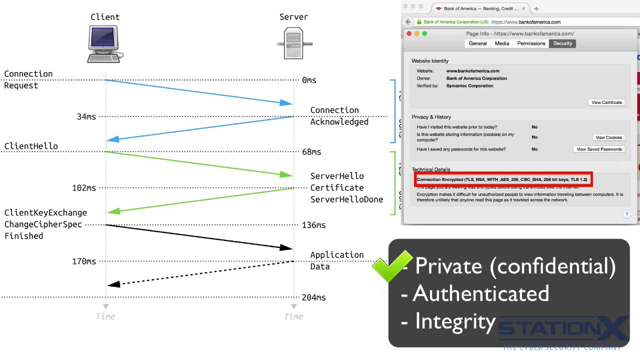 even by an attacker who places himself in the middle of the connection. The connection is also reliable because the encryption is used to encrypt the data transmitted. This in that no attacker can modify the communication during the negotiation without being detected. The identity of the communicating parties can be authenticated using public key cryptography. 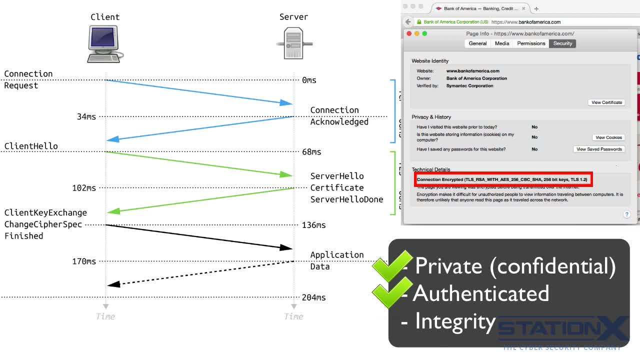 certificates and digital signatures. This authentication can be made optional, but is generally required for at least one of the parties, usually the server, so the websites you visit, And I'll show more on this. when we talk about certificates, The connection is reliable because each message transmitted includes a message integrity check. 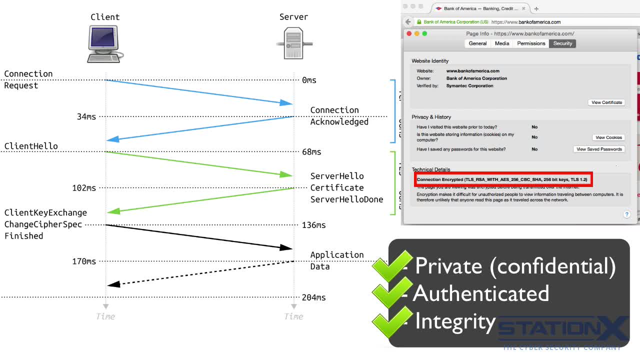 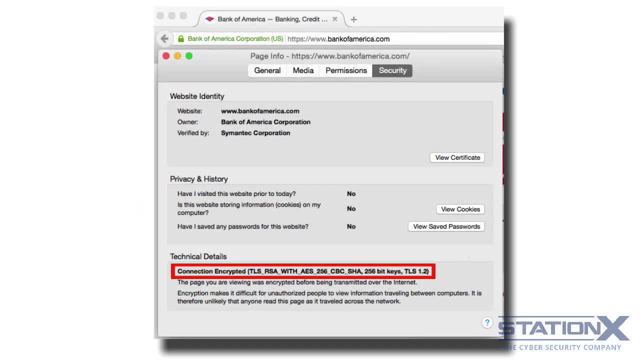 using a message authentication code, or MAC, to prevent undetected loss or alteration of the data during transmission. TLS supports many different methods for exchanging keys, encrypting data and authenticating message integrity- many of the algorithms and technologies which we've already discussed. 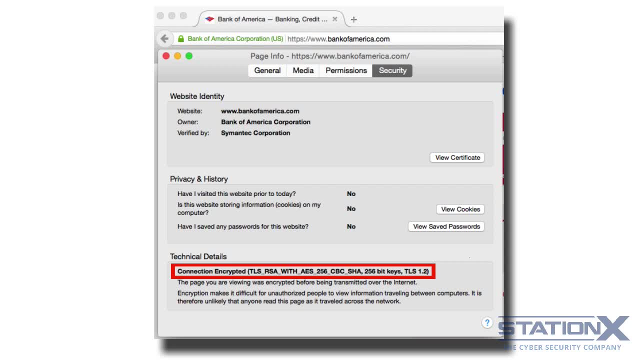 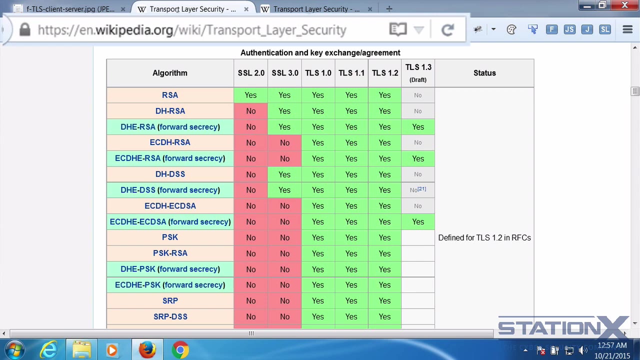 As a result, though, secure configuration and the authentication of TLS involves many configurable parameters, and not all choices provide the security services of privacy, authentication and integrity. Now, if we look on the Wikipedia site for transport layer security, which is actually a brilliant site for describing TLS, 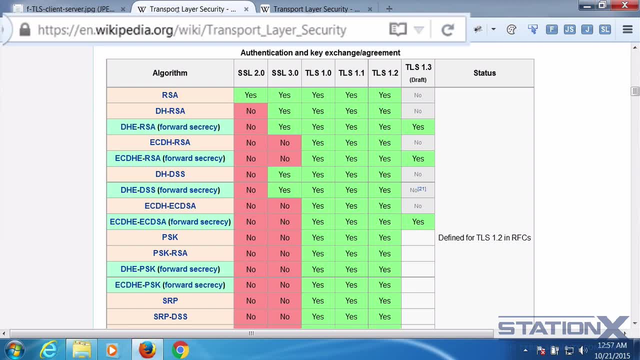 we can see the various different supported methods for exchanging keys, encrypting data and authenticating message integrity, And the first one here is showing us authentication and exchanging of keys in the various different algorithms that are supported. Now, if you remember back to the asymmetric algorithms that we discussed, 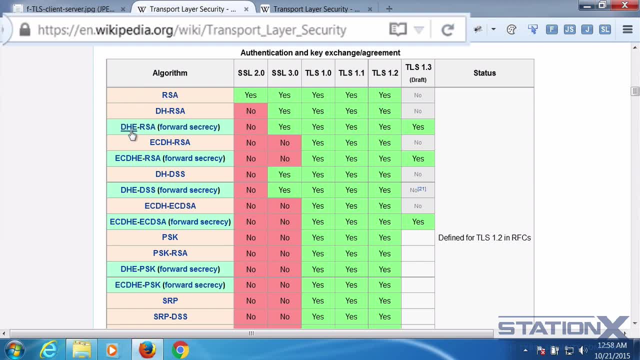 that's these. so we can see RSA, we can see Diffie-Hellman RSA, elliptical curve, etc. Now the best ones to use are this one and this one and this one. But the problem is you don't always get a choice. A server will. 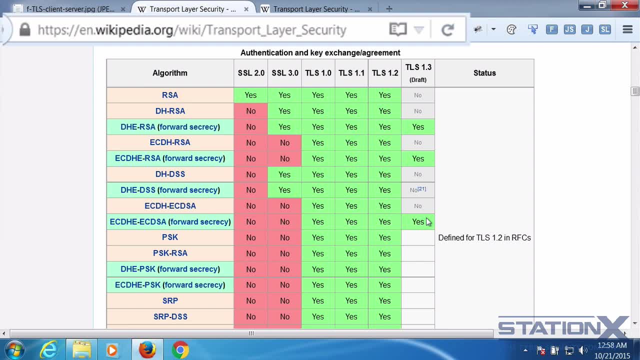 support certain authentication and key agreement methods and if you want to speak to them, then you'll have to use those. Now, the reason that these are the preferred option is because they're using Diffie-Hellman for key exchange, which can ensure a property of privacy called forward secrecy, which you can see. 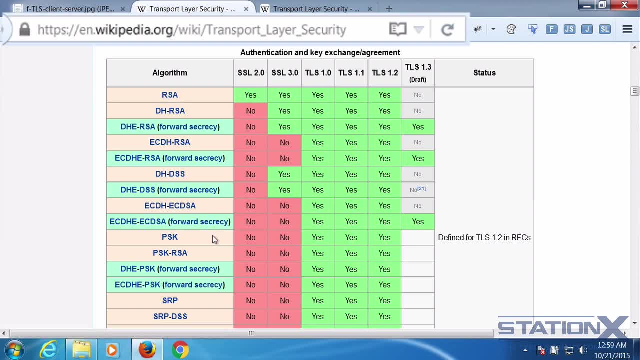 here Now. this property gives assurance: your session keys will not be compromised, even if the private key of the server is compromised, By generating a unique session key for every session a user initiates. even the compromise of a single session key will not affect any data other than that exchange. in that, 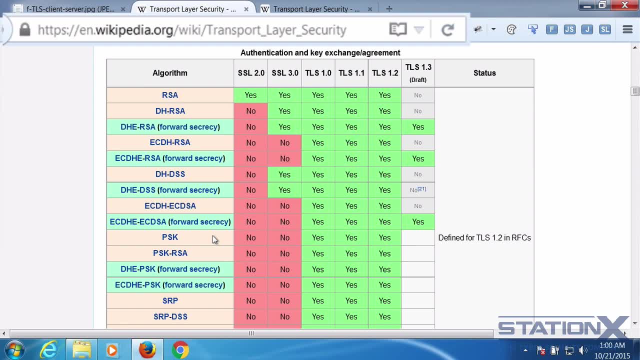 specific session protected by that particular key. Perfect forward secrecy represents a big step forward in protecting data on the transport layer and has become to see more important since vulnerabilities such as heart bleed. So perfect forward secrecy really means that if the server you're communicating with is compromised, and their private 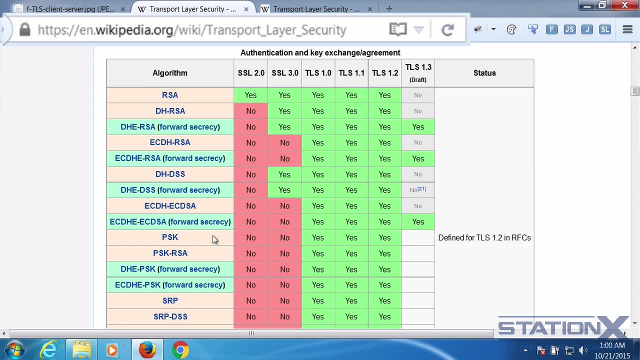 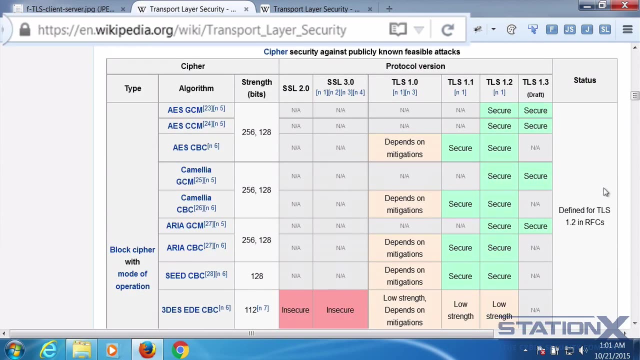 key is compromised, it means that all of your previous conversations cannot be decrypted, because you're using Diffie-Hellman to negotiate session keys that are only used for a very short time. If we move further down on here, we can then see the symmetric algorithms that are used. So when we're 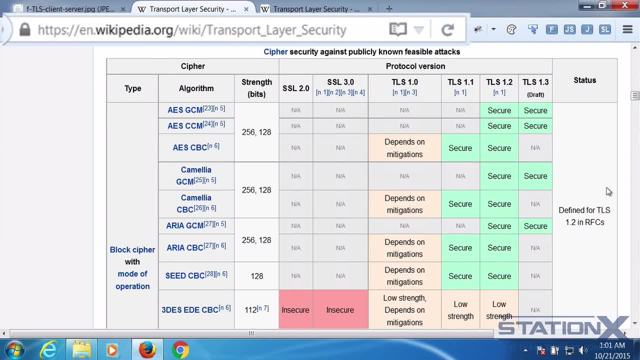 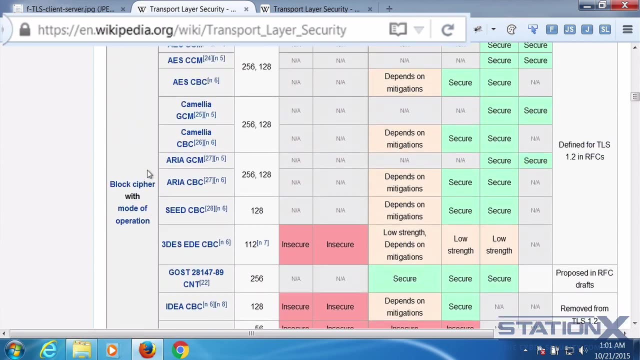 talking about session keys. these are the keys that are actually used to encrypt the data, because the symmetric keys are quicker and remember, we talked about AES and now AES was a good option, and here we can see AES and various other types of symmetric encryption algorithms, and this interestingly shows us which one. 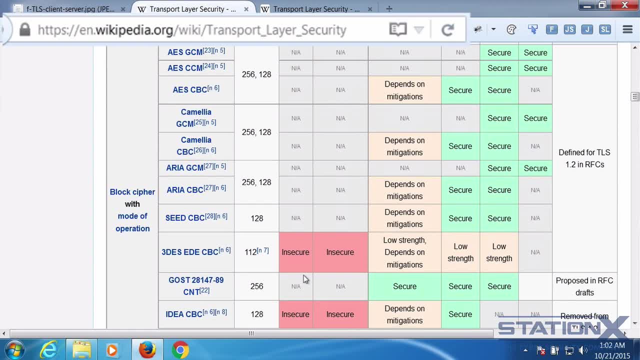 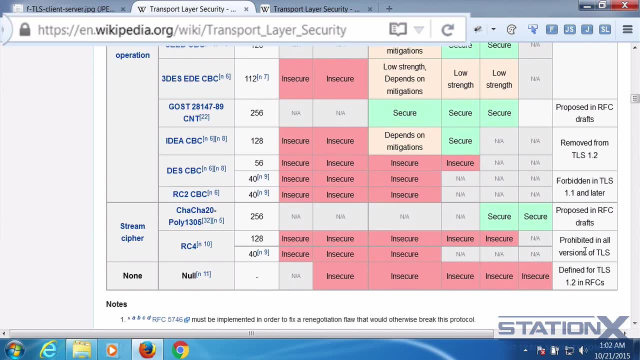 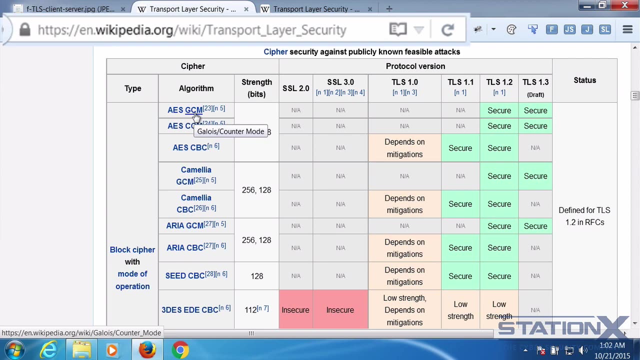 are secure and which ones are insecure, That'll be because there's some sort of vulnerability or weakness against them, which is another reason why I recommended AES. You'll notice here that there are some other things at the end of this AES. You shouldn't really worry too much about that. That is called a. 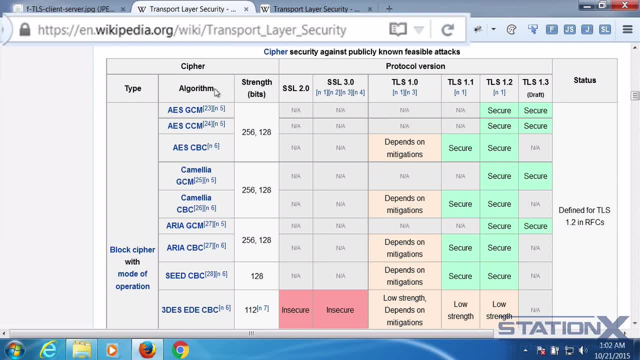 mode of operation. It is a different way for AES to scramble or encrypt the data, which doesn't really matter too much in this case and for this course, Just knowing that you're using AES is enough, and the bit length which we've already explained You can also see here. it illustrates the different versions of 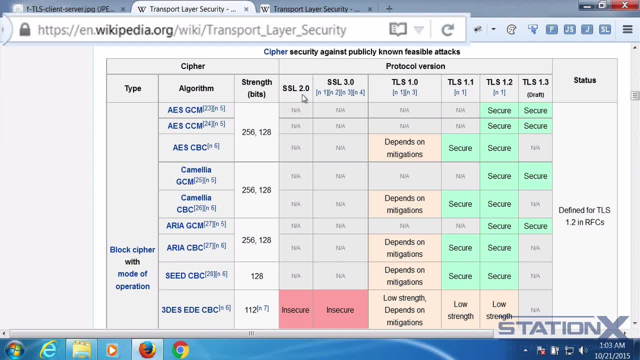 SSL. So actually- and this is very confusing for a lot of people- this is the first version, or earliest version that it's showing here, of SSL, and this is the next one, and then this is the next one, So it goes to 1 after it was at 3 for SSL. So TLS 1.3 is the latest and most secure. 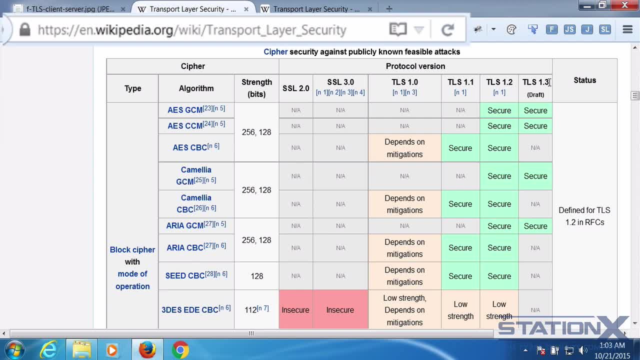 version but is the least compatible with browsers. So when using TLS you really want to be on TLS 1 or above, As you can see here. you can see which one of these is secure or not secure and you can see here. even with AES you've got depends on. 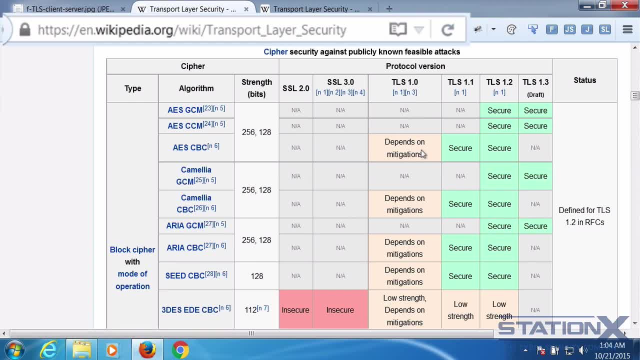 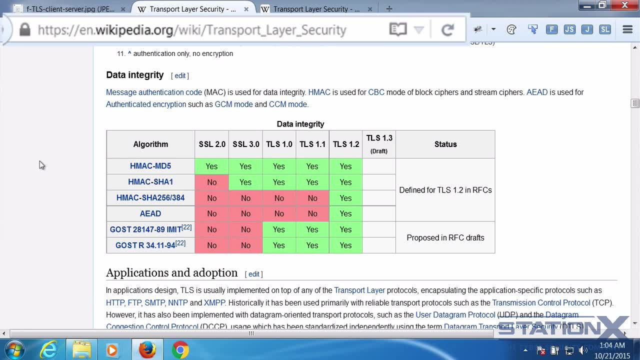 mitigations if you're using TLS 1.. Let's come down a little bit further and you can see the hashes and MACs that are used in order to maintain data integrity. MD5 shouldn't be used. SHA-1 is definitely getting very old and we. 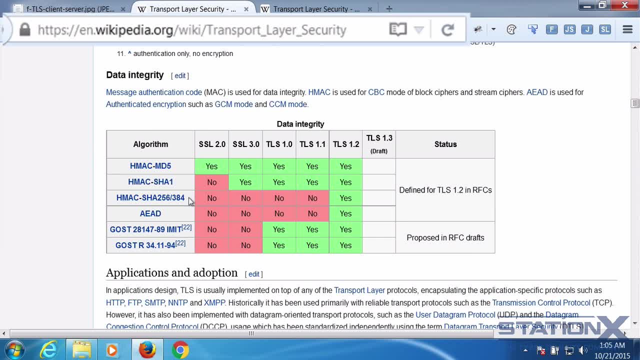 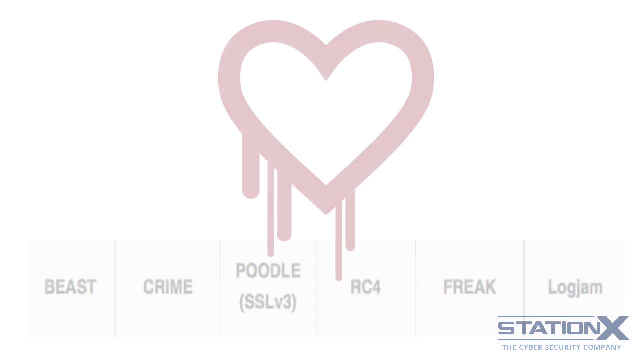 should be starting to use the later versions of SHA, which is 256 and 384, but for compatibility reasons these aren't necessarily used. Attempts have been made to compromise and subvert aspects of the security. that TLS and the protocol has been revised several times to address these evolving security threats and identified weaknesses. 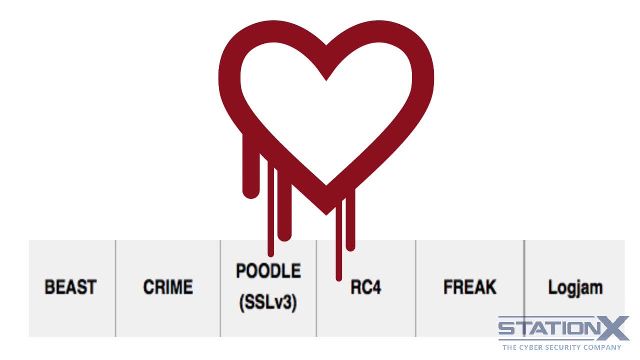 and vulnerabilities. Examples of these include Beast Crime, Poodle, Logjam- all with interesting names. You can Google those and find out more details if you're interested. but the result of the server implementations of SSL has had to be upgraded by the developers in order to keep. 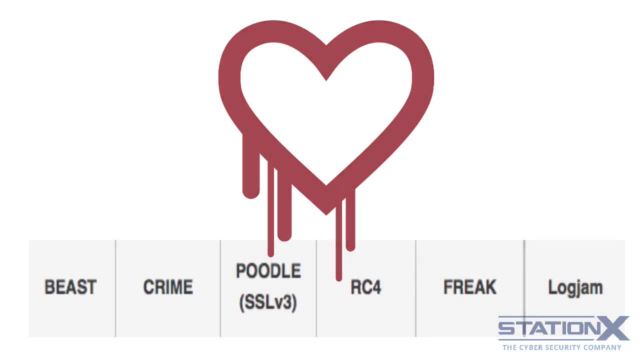 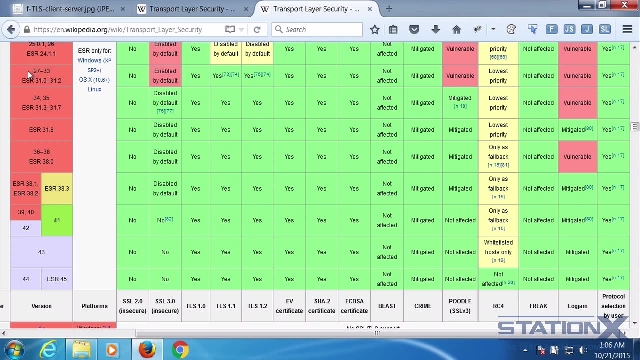 up with the attacks and to defend against these vulnerabilities. Now, if we go here, you can see listed the versions of Firefox. this is Firefox 27 to 33, and you can see Beast Vulnerability, Crime, Poodle Free, and the last one is the one of the most common ones. 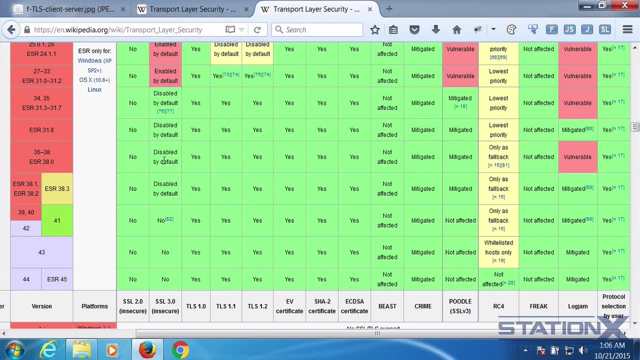 Freak Logjam and you can see if you've got version 36 to 38, then that is vulnerable to logjam and if you get older and older versions, you'll see that they become more and more susceptible to various weaknesses and vulnerabilities, which is why you should be on the latest version of your browser where possible. 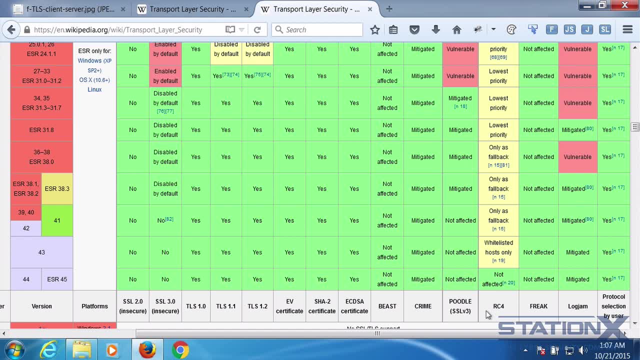 and the servers or sites that you connect to also need to be on the latest versions. and the thing is, you can't necessarily control that. but the thing is, if you need privacy, you need extreme privacy, and you know that your server is not supporting or is vulnerable to some of these things because maybe it's using 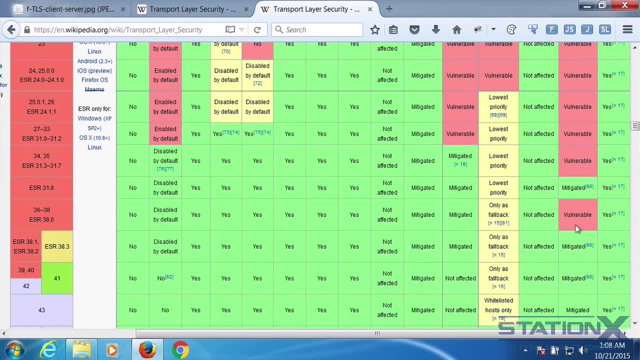 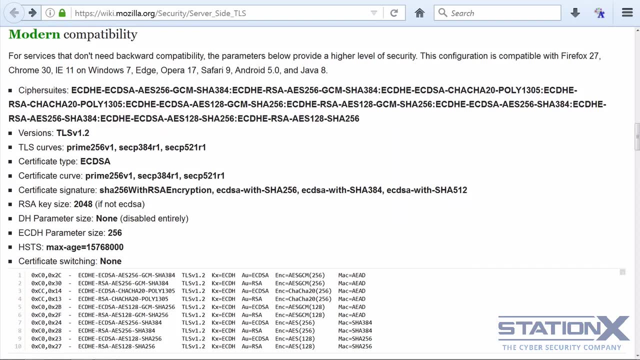 just SSL one, then you know that you can't communicate with that, not in a secure and private way. The combination of algorithms used is known as a cipher suite. It is useful to know what are both the strongest and most compatible cipher suites. So instead, 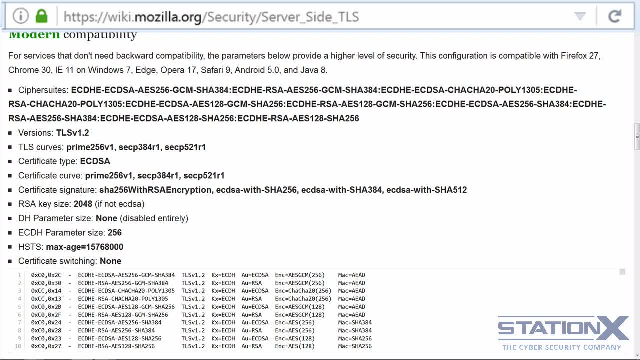 of giving you a list, I'm going to point you at resources that you can use instead. This way, you can find the latest cipher list to be considered the most secure and compatible when you need it. This is because, if I give you a list now, 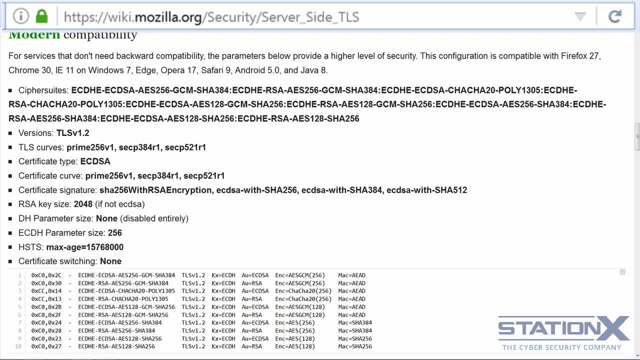 tomorrow a new vulnerability could come along and you'll be able to access it. This is because, if I give you a list now, tomorrow a new vulnerability could come out which would invalidate the order. Probably one of the best places to go for a good cipher suite with compatibility- well, actually the best. 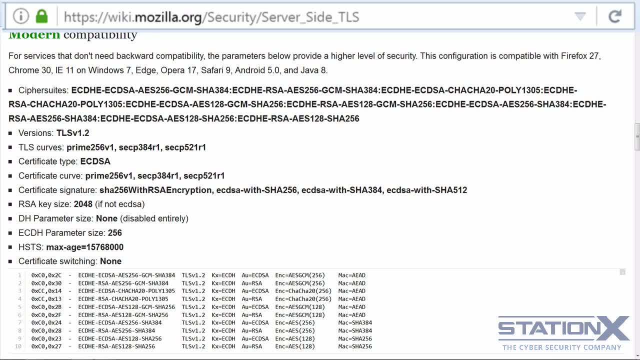 place I know of anyway, is Mozillaorg, the people behind Firefox. Now, what you can see here is the cipher suite list in order of preference. So here is the most desirable and here is the least desirable. The cipher suite is very simple but still strong. Plus, you have all of the best. 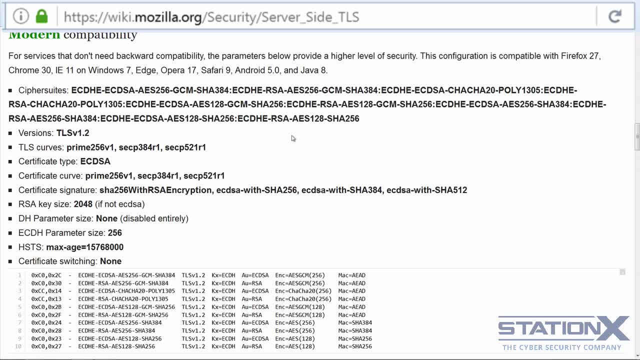 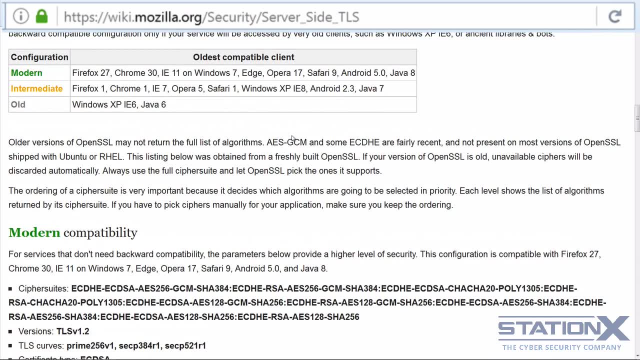 options as well, such as your TLS version, your certificate type, your certificate signature, etc. And if you go up here, you can see what these ciphers are compatible with. So these are the oldest compatible clients that will work with these ciphers. So that's a really great list of the strongest ciphers, the ones 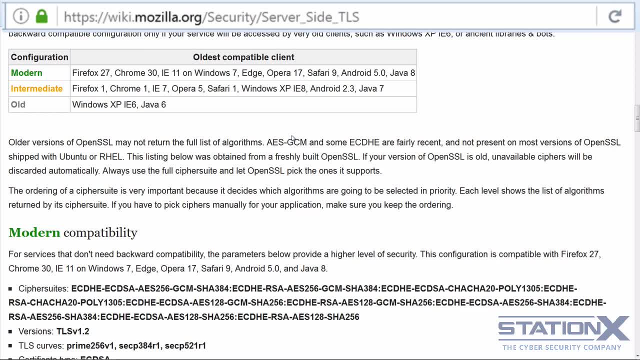 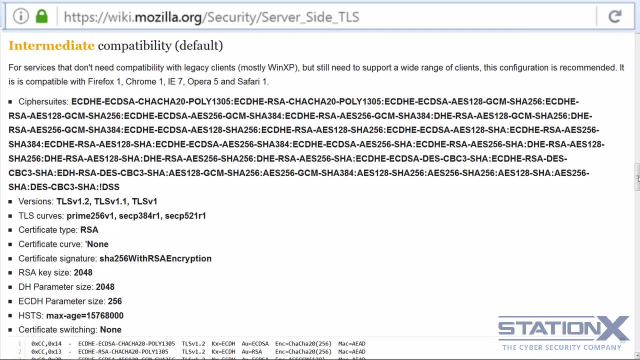 that you want to use in preference, And also, if we go further down here we have a list designed for increased compatibility. So if you're looking for a list that'll work with a wider number of clients, then this is a good option here. If we go further down, there you go they. 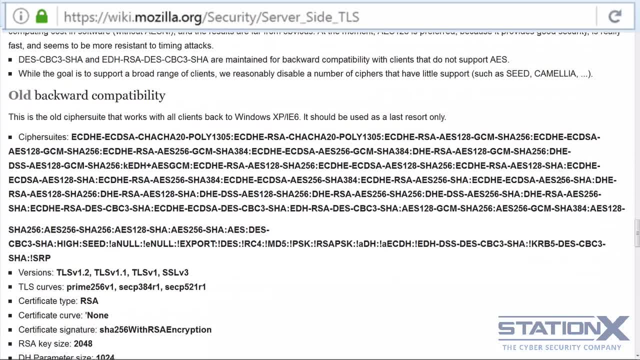 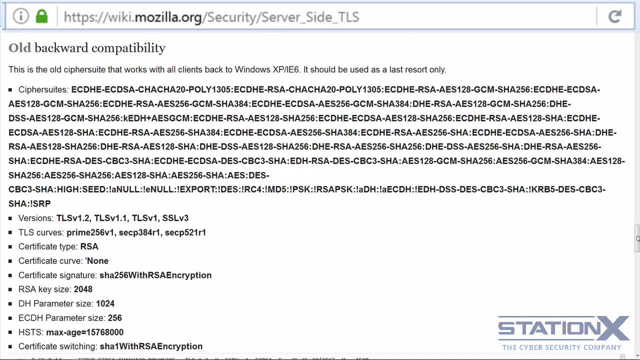 see all the ciphers. If we go further down we can see like the ultimate compatibility list here which will work with the really older clients. If you need to configure a server, then check this out. this is a really cool tool. so if we select the type of